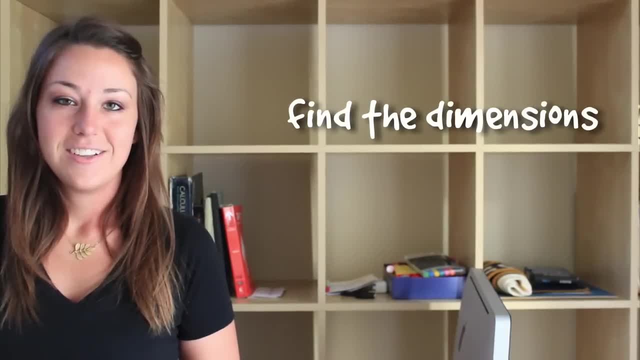 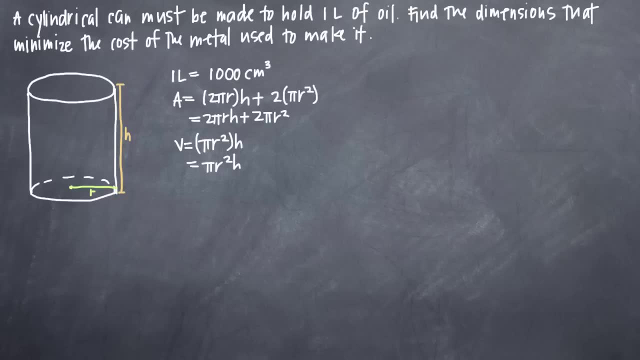 derivative of the optimization equation to find the dimensions. Let's take a look In this particular optimization problem. we've been told that a cylindrical can must be made to hold one liter of oil, and then we've been asked to find the dimensions of the can. 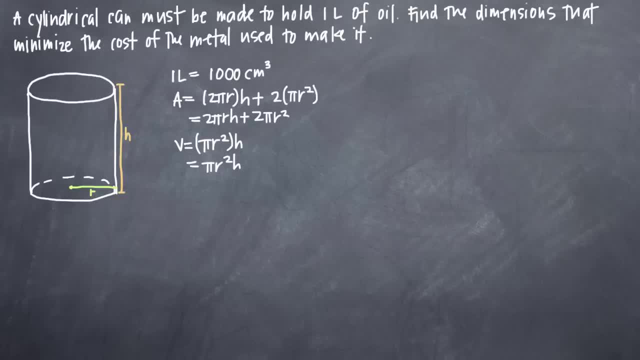 that will minimize the cost of the metal used to make it. As with any optimization problem, the first thing you want to do is draw a diagram of what you've been told and write down as much information as you can. So we've drawn a diagram of the cylinder and we've 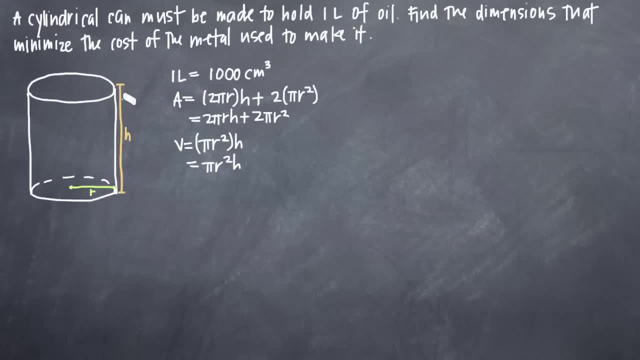 indicated r as the radius and h as the height of the cylinder. We've also written down that one liter is equal to a thousand cubic centimeters and that the area formula for a cylinder is 2 pi r h plus 2 pi r squared. We also know that the volume of a cylinder is pi r squared. 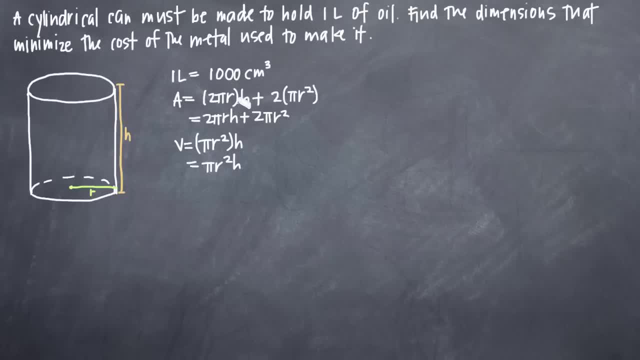 h. So really quickly, in case you don't remember those, remember that the area formula is 2 pi r, which is the circumference of the circle times h the height of the can. so that gives you the outside or the material used to make the side, And then pi r squared is the area. 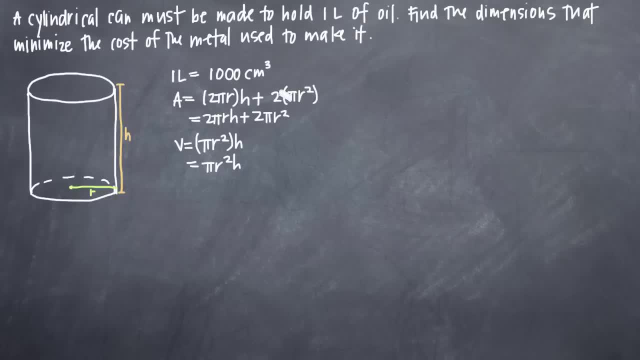 of the circle, so that will give you the top and bottom. You multiply by 2 and you get 2 pi r h plus 2 pi r squared. The formula for the volume is the area of the circle times the height of the can, So the area of the base times the height, which will give us the 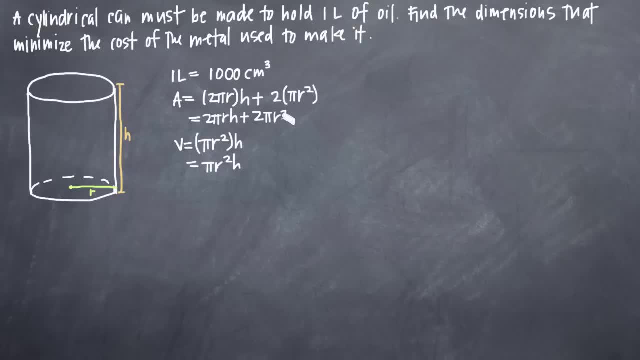 total volume of the can. Once we've written down all the information that we've been given, our next step is to identify a constraint equation and an optimization equation. So with any optimization problem like this, you are always going to need an equation that has a maximum value of 0.5.. 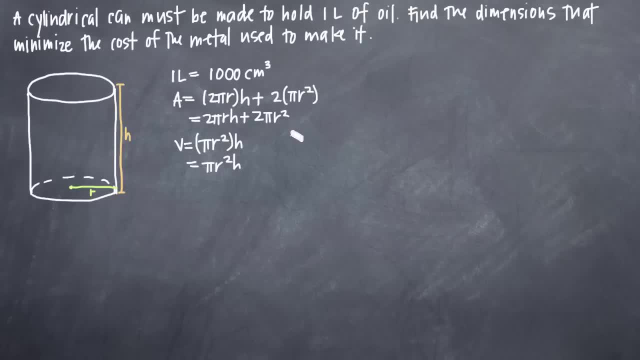 equation you can optimize, but you'll also need a constraint equation, Because we've been asked to minimize the cost of the metal. that means that we're going to be minimizing the surface area of the can, because the metal is defined by the surface area. So minimizing 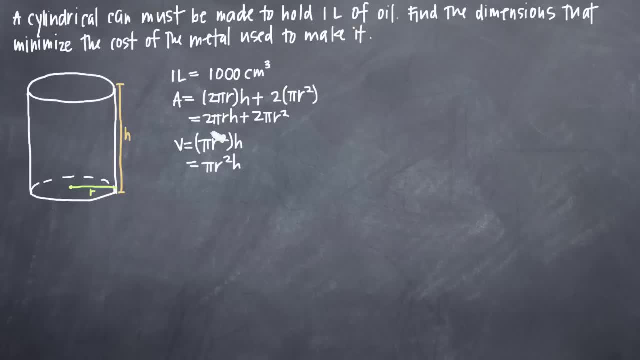 the surface area means that our optimization equation will be the area equation. So let's go ahead and just say that this area equation here will be our optimization equation. Our constraint equation is the equation that limits us. So we've been told that the cylindrical 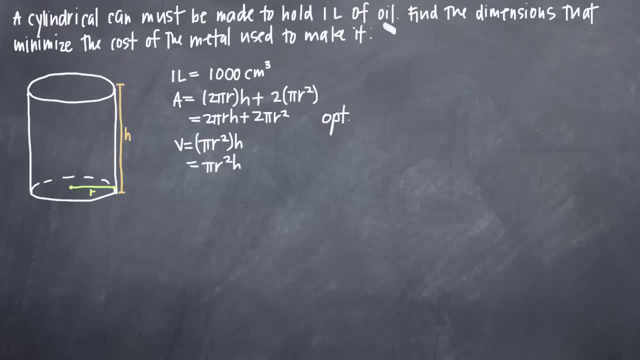 can has to be made to hold one liter of oil. That's the only constraint we've been given. So what the problem is asking is for us to optimize the area, the surface area, minimize the cost of the metal or minimize the cost of the surface area within the constraint. 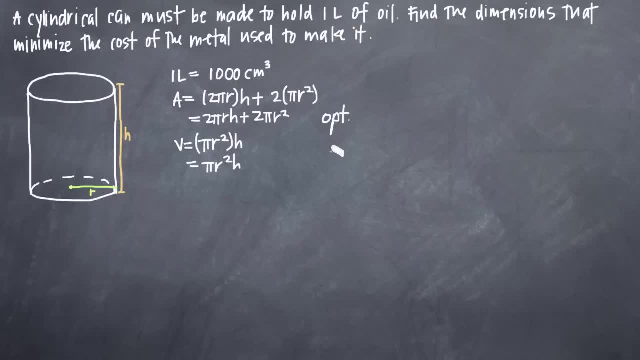 or within the condition that the volume has to hold one liter or 1,000 cubic centimeters. So this volume equation is going to be the constraint equation that we're going to be solving. So the constraint equation here will be our constraint equation. Our next 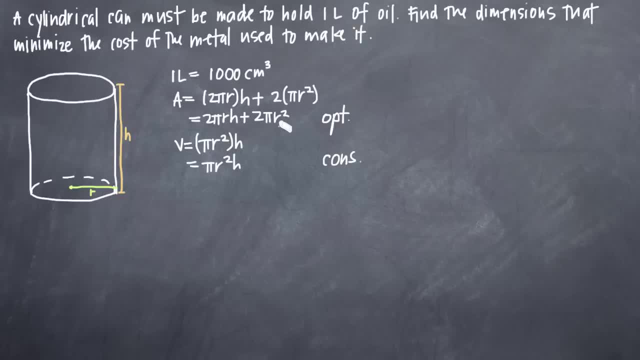 step is to figure out how to reduce our optimization equation to just one variable. So because we have in our optimization equation here both r for the radius and h, we need to get rid of one of those. The way that we're going to get rid of one of them is by solving the. 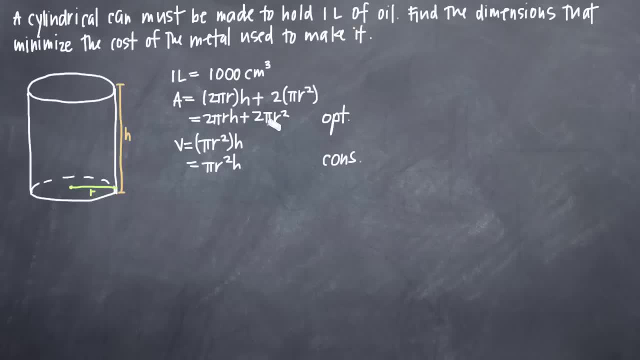 constraint equation for one or the other and then plugging in to the optimization equation. So let's go ahead and solve our constraint equation, our volume equation, by just using the r squared or h In this case. let's go ahead and solve it for h, because that'll be. 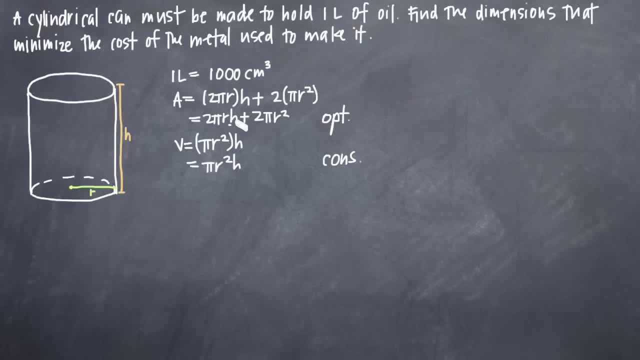 really easy to plug in to the area equation. We've just got h right here. So the way that we'll do that is by plugging 1,000 cubic centimeters in for volume- We know that has to be the volume- And we'll set that equal to pi r squared h and then we'll solve for h, Obviously to. 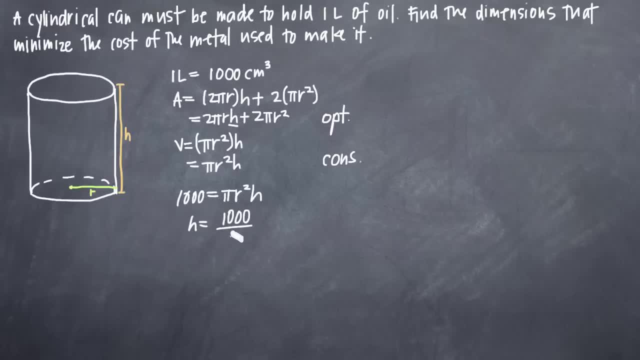 solve for h. we'll just divide both sides by pi r squared And then we'll just plug in to the area equation. We've just got h right here. So the way that we'll do that is by plugging in 1,000 cubic centimeters in for volume. We know that has to be the volume. 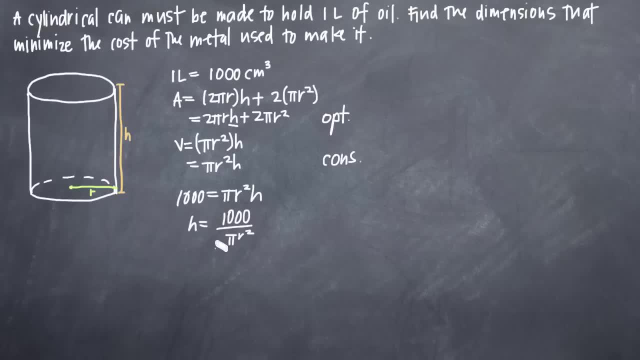 So we'll get 1,000 divided by pi r squared. Now that we've solved for h, we can go ahead and plug that back into our area equation. So if we say area over here is equal to 2 pi r multiplied by h, which we solved for as 1,000 over pi r squared plus 2 pi r squared, 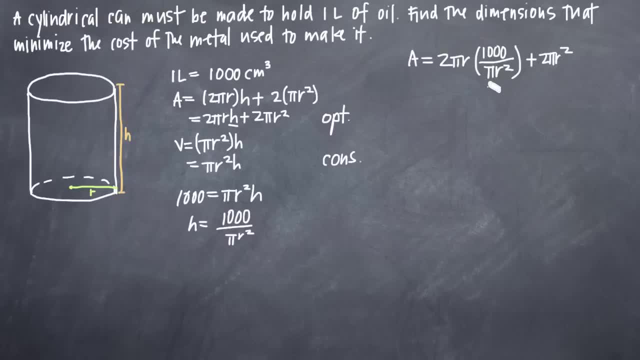 Now we have our optimization equation for surface area in the form of h, So we're going to have our solution in the form of a respect to 1 pi r squared, And so we'll go ahead and plug in 2 squared h squared into b, And that is equal to h times pi r squared plus 2 pi. 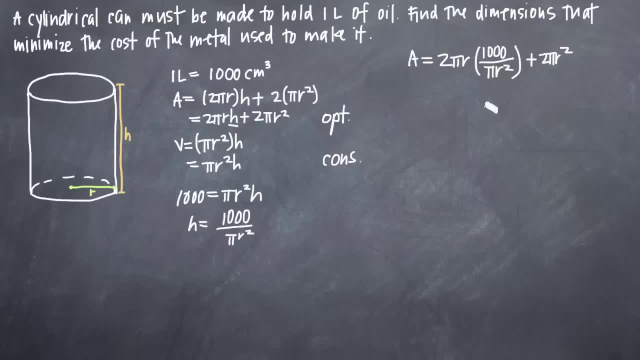 r squared plus b squared, which is equal to 2 pi r squared. So we'll plug in 2 and then we'll get 1,000 over pi r squared. So that's the value of the solution. Now we only have 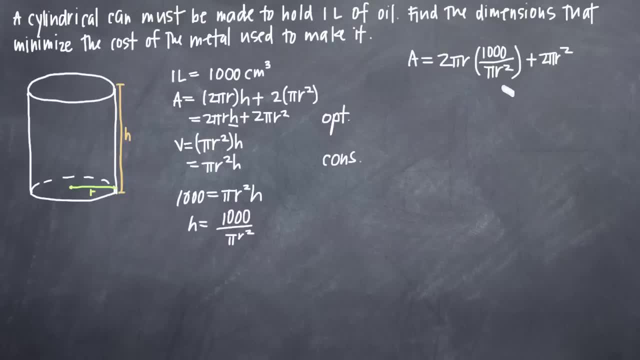 to plug in 1,000 over pi r squared, And then we'll plug in 2, and then we'll plug in 1.. So now that we've got it in 1 variable, all we need to do is simplify. take the derivative. 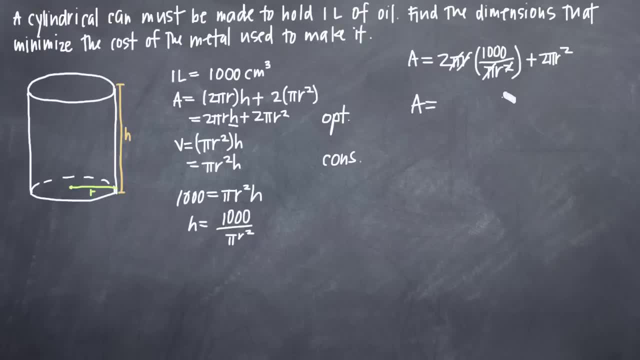 set the derivative equal to 0, and solve for r And r should give us the radius of the can that minimizes the surface area, r plus 2 pi r squared. Now we need to take the derivative, because we've simplified this as much as possible, So let's go ahead and make this a little bit easier on ourselves. 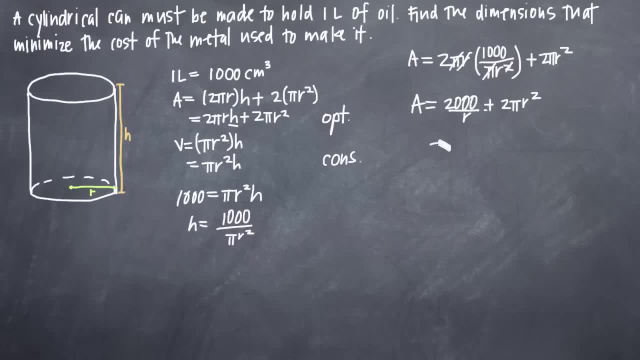 We'll call this 2000r to the negative 1.. Remember that we can move a variable from the denominator to the numerator just by changing the sign of the exponent from a positive to a negative. So 2000r to the negative. 1 plus 2 pi r squared. If you're not comfortable doing this, you 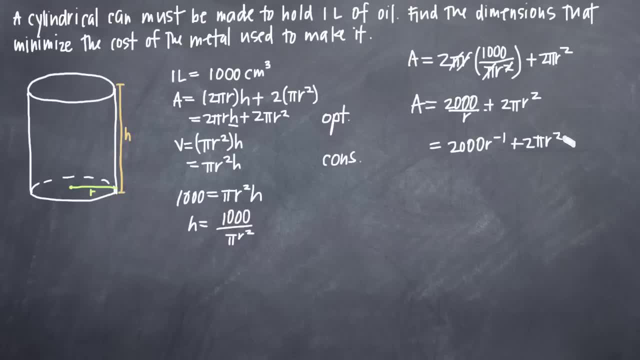 can obviously use quotient rule to figure this out. So we're going to take the derivative a prime and we'll get negative 2000r to the negative 2 plus 4 pi r, And when we move this to the numerator we're going to get negative 2000r to the negative 2 plus 4 pi r squared. 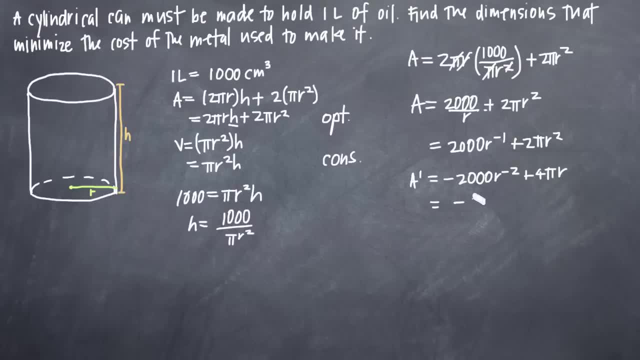 So we're going to take the derivative a prime and we'll get negative 2000r to the negative 2 back to the denominator, We'll get negative 2000,. and actually let's go ahead and make that our second term, so we don't lead with a negative. We'll get 4 pi r minus 2000 over. 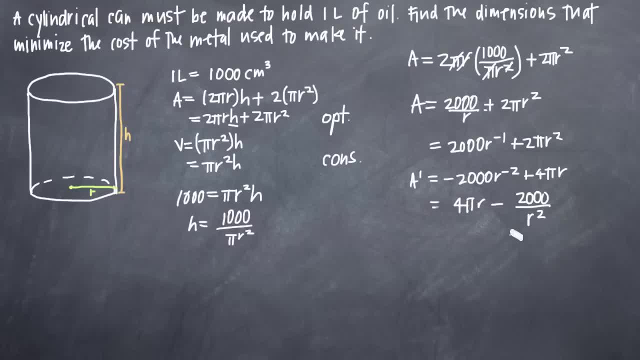 r squared. So that is our derivative equation. Now we need to set this equal to 0 and solve for r. So if we set it equal to 0, let's at the same time go ahead and find a common denominator. In order to find a common denominator, we're going to be multiplying this first term by 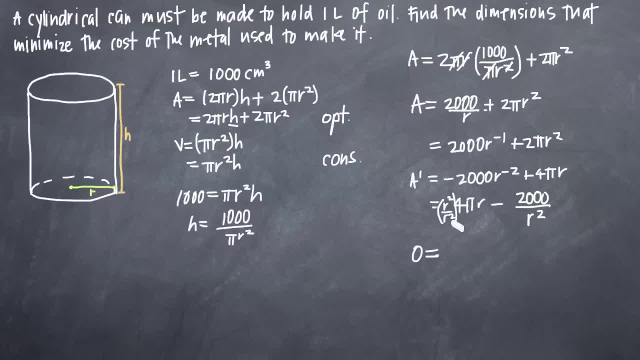 r squared over r squared And we'll get 4 pi r cubed. We can combine the fractions Minus 2000 all over r squared. So now what we can see is that this right-hand side here is going to be equal to 0 whenever the numerator is equal to 0 or if the denominator is undefined. 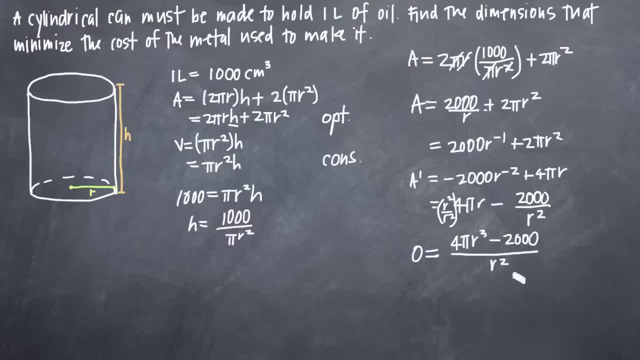 However, if the denominator is undefined, that means r is equal to 0. And we know r can't be equal to 0 because we're talking about a three-dimensional figure here in real space. and if r is equal to 0, then the cylinder doesn't exist. So we can almost just discount. 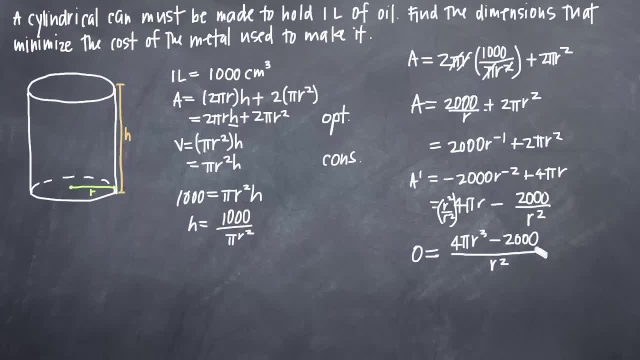 that, and we're really just looking at where the numerator is equal to 0. So let's go ahead and factor out a 4, and we'll get 4 times pi r cubed minus 500.. Obviously now we can see that the right-hand side will equal 0 only when pi r cubed minus 500 is equal to. 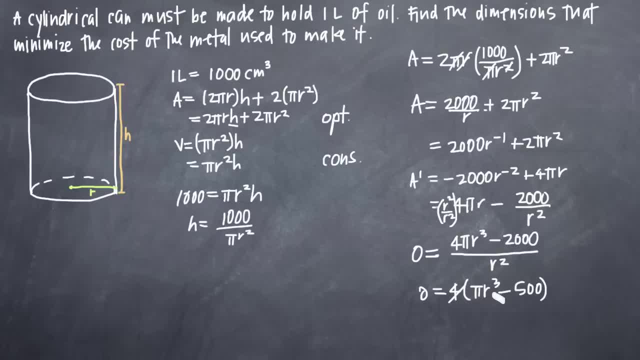 0. So we can really just ignore the 4 or divide both sides by 4, and that'll go away. And now, if we add 500 to both sides, we'll get 500 equals pi r cubed If we divide both sides. 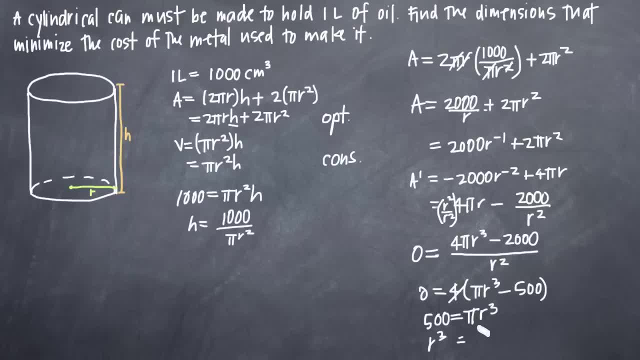 by pi, we'll get r cubed equals 500 divided by pi. And if we solve for r by taking the cube root of both sides, we'll get r equals 0. So we'll get r equals the cube root of 500 divided by pi. We know now that this must 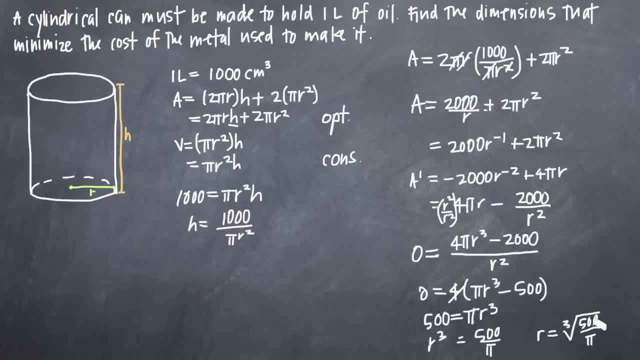 be the radius. that minimizes the surface area of the can. If we want to find the height as well, we can just go ahead and plug r into our height equation. It's not very clean, but we'll get 1000 divided by pi times, and now we have r squared here, so we get the. 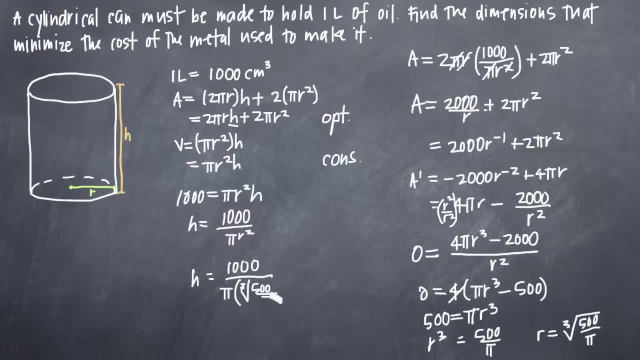 cube root of 500 divided by pi. And now we can see that r squared is equal to r cubed over pi times 500 over pi to the 2 thirds power. So these are the dimensions- h here and r here, that minimize the surface. 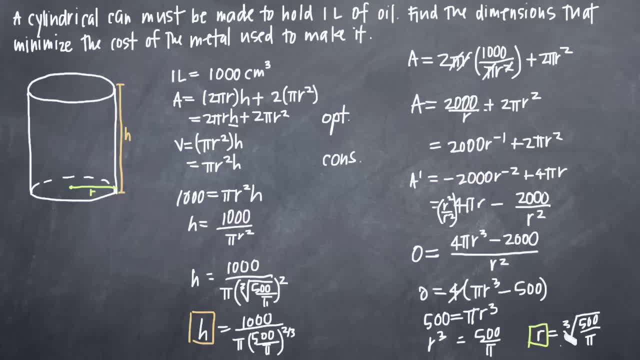 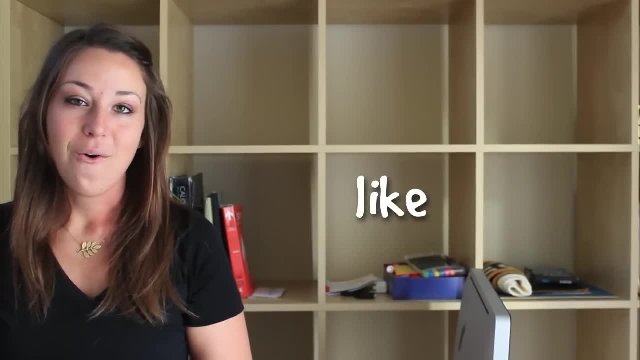 area and therefore minimize the cost of the metal used to construct this. So now we can just go ahead and plug r in …. check the can. So I hope you found that video helpful. If you did, like this video down below and subscribe to be notified of future videos.